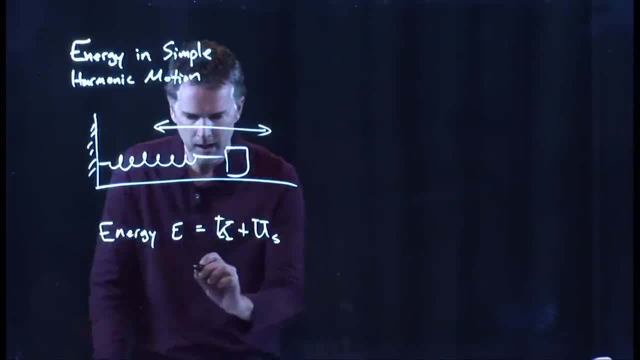 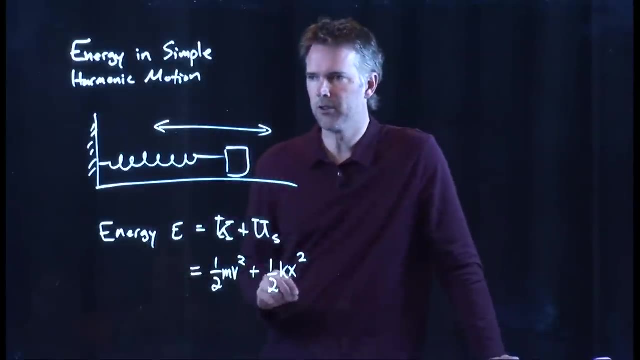 Okay, but we know a little bit about that stuff. right, We know that kinetic energy is one half mv squared And we know that spring potential energy is one half kx squared, where x is how far you stretch the spring from its equilibrium position. 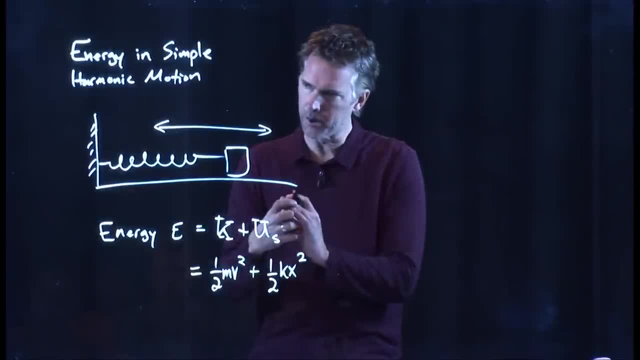 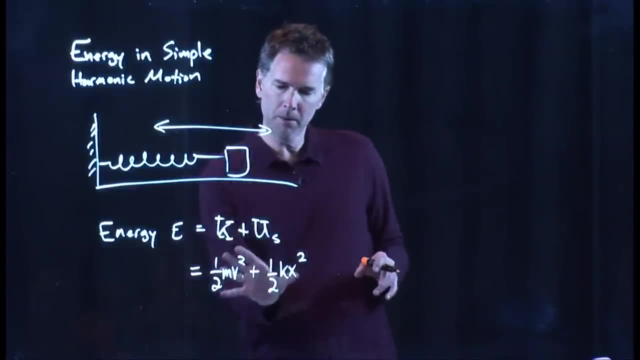 Since it's squared, you would get the same answer if you compress the spring by the same amount. It doesn't matter that it's a negative. once you square it it becomes positive. Okay, that's good, but we know a little bit more about those for simple harmonic motion, right? 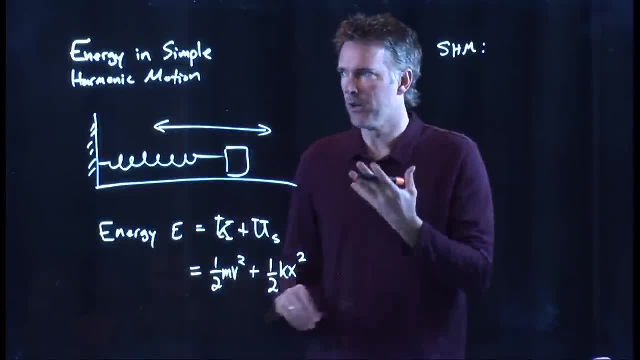 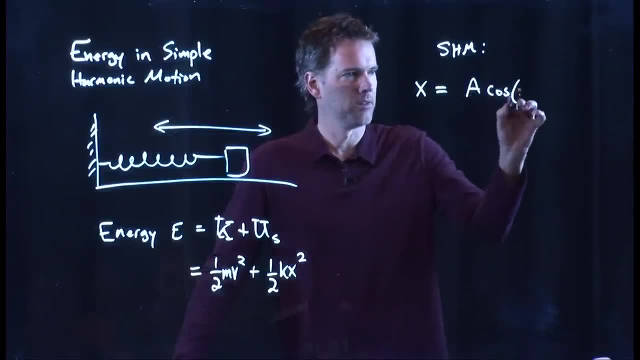 So we wrote down the differential equation for simple harmonic motion and what we discovered was x has a particular solution. we can write it like this: a cosine, omega, t plus v, And if that is x, then we can get v very easily by taking the derivative of x, and when we do that cosine becomes negative sine. 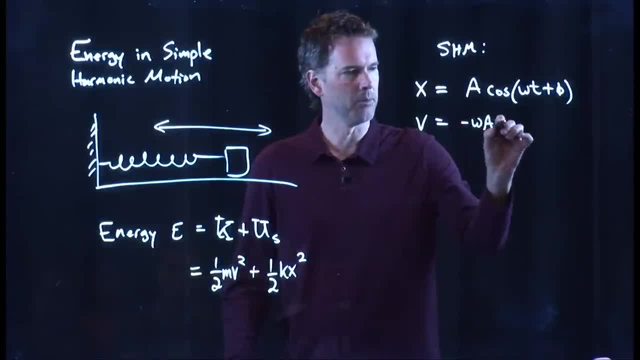 I have to pull out an omega from inside the argument, and so v is this negative omega a sine of omega, t plus v. And now I can put all that back into this equation. So what does energy become? One half m times v squared? Here's my v, right here. 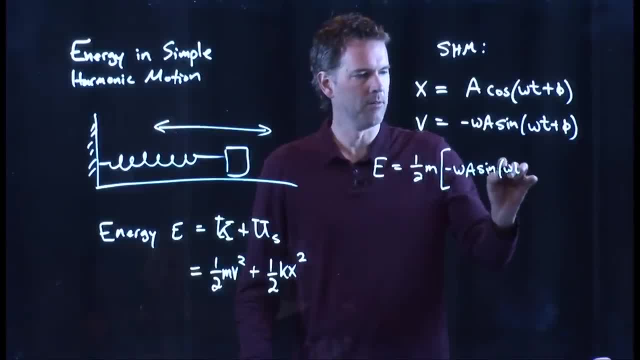 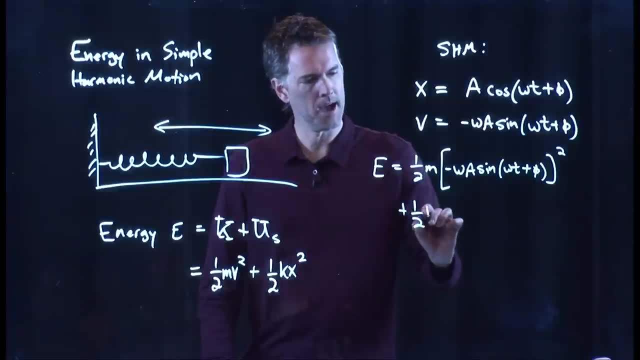 Negative omega a, sine of omega t plus v. We're going to square that, And then we're going to m times v squared, And then we're going to m times v squared, And then we're going to add one half k times x squared. but there's my x. 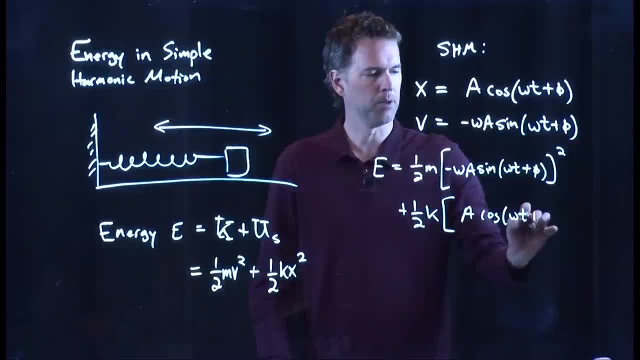 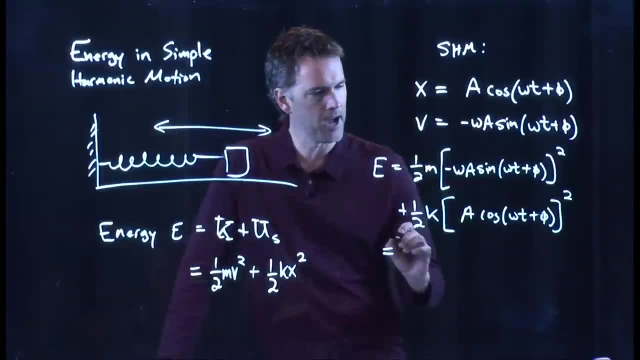 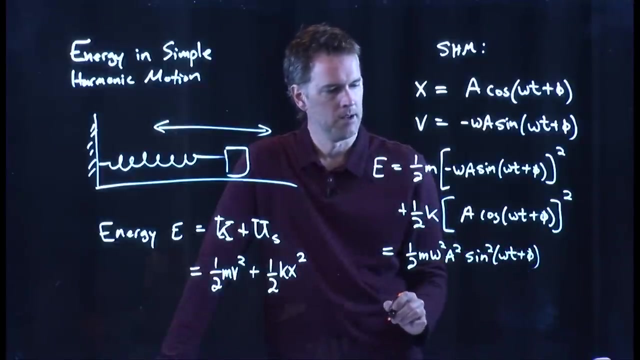 A cosine, omega t plus v, quantity squared. And now we can write out this stuff right: We've got one half m omega squared, a squared times sine squared of omega t plus v. And then the next one is one half k, a squared cosine squared omega t plus v. 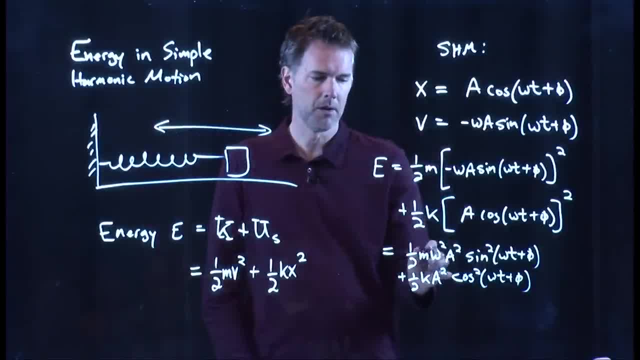 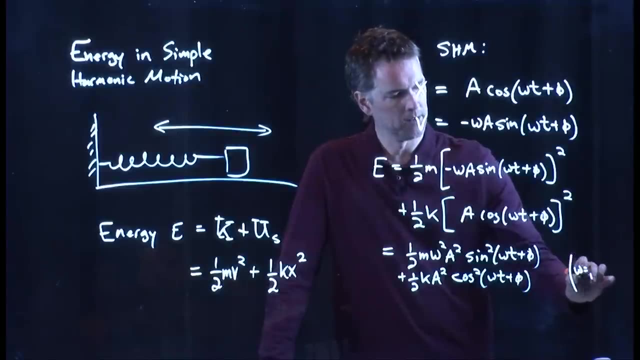 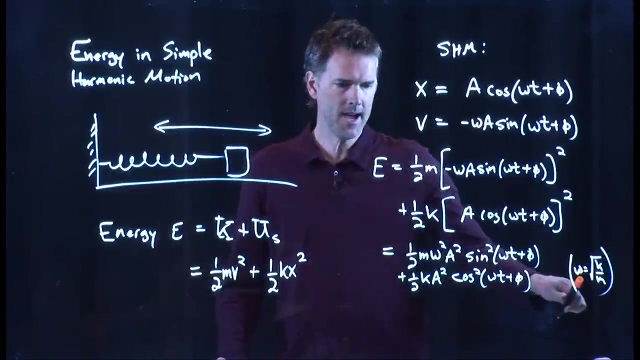 And it looks like maybe we can't combine those unless we remember that omega is in fact related to k. That was one of those things that we derived before. Omega is, in fact, the square root k over m, And if omega is that, then omega squared just becomes k over m. 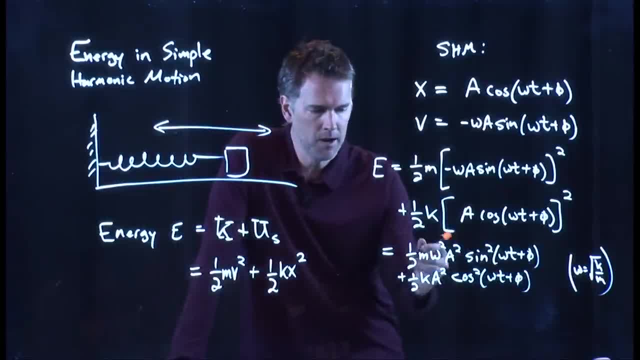 And if omega squared is k over m, that m cancels out and I get one half k a squared on both of those terms And I get one half k a squared on both of those terms. That term becomes one half k a squared And that term was already 1 half k a squared. 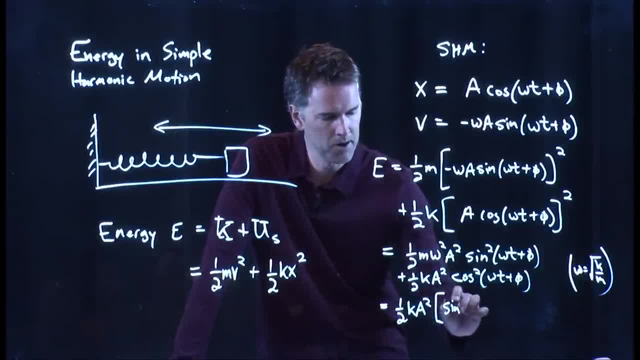 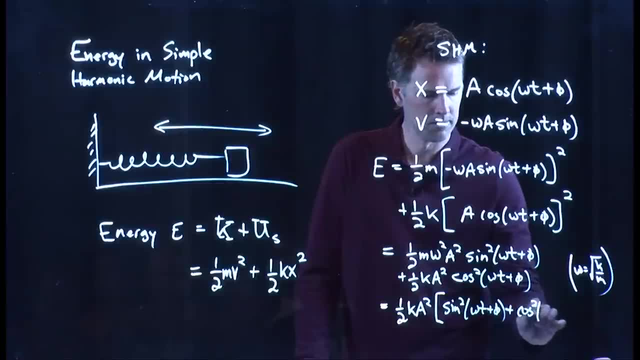 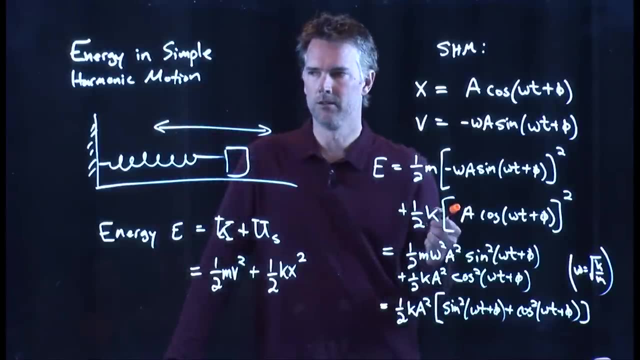 And now everything that's left is just sine squared omega t plus phi, plus cosine squared omega t plus phi. And now we go back to our joke, right? Anybody remember the joke? What's the geek pickup line? Right? Geek approaches the girl at the bar and he says: 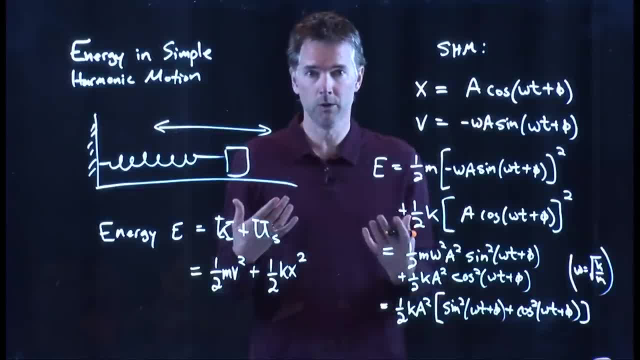 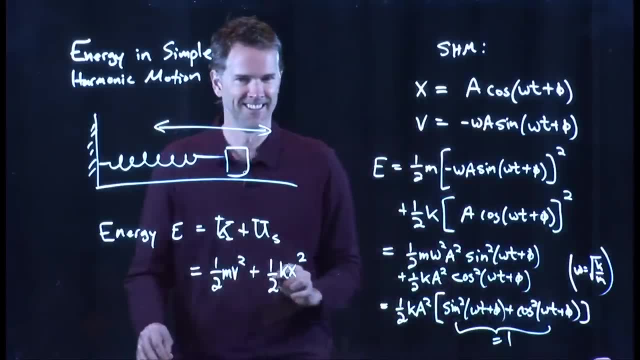 I wish I was sine squared and you were cosine squared, so together we could be 1.. You are allowed to boo in here if you want. That's fine. That is equal to 1.. And so look the total energy. what does it simplify to? 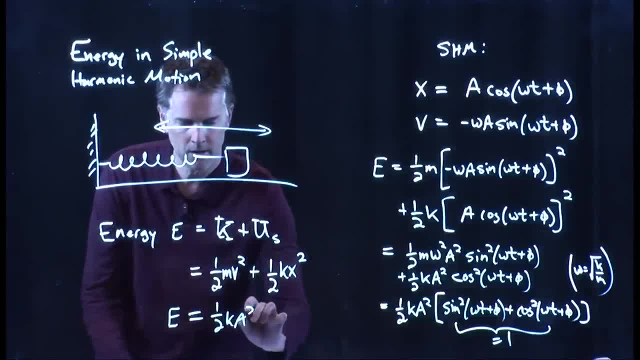 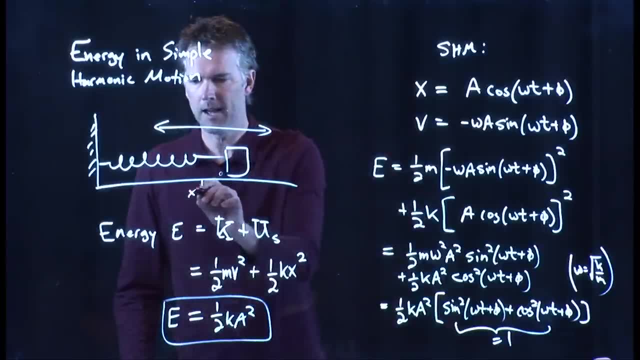 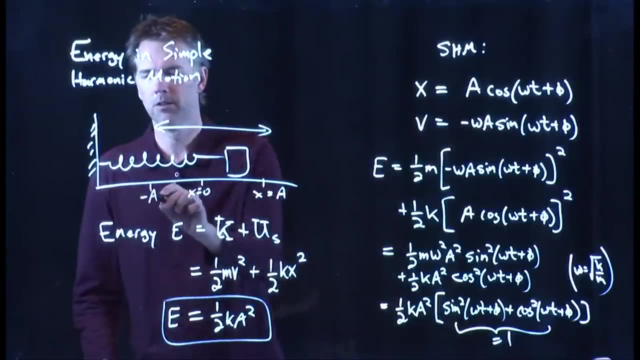 1 half k a squared, That's it. That's the total energy in the system. However, far So, if you stretch this thing out from x equals 0 to x equals a and you let it go, that determines how much energy is in the system. 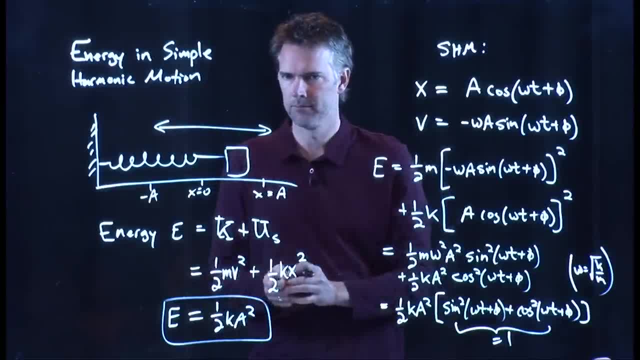 At full stretch. it's all that Okay, And that is of course, a constant. K is a constant, A is a constant, And so it doesn't change as a function of time. The total energy of the system is fixed. Okay, That's it. It's fixed as a function of time.